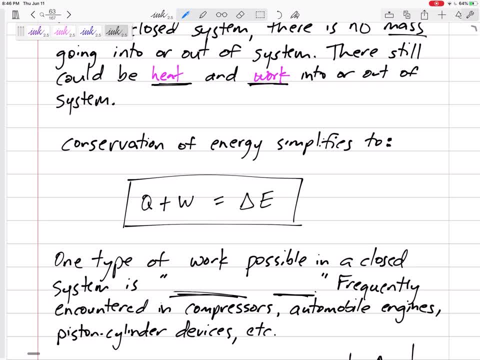 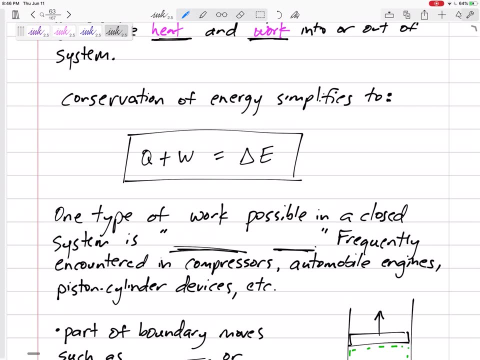 If it's out, it's negative And equals change in energy. That change in energy could be potential energy, kinetic energy, flow work and internal energy right there, Okay. so the very first section- 4-1, is all about boundary work. 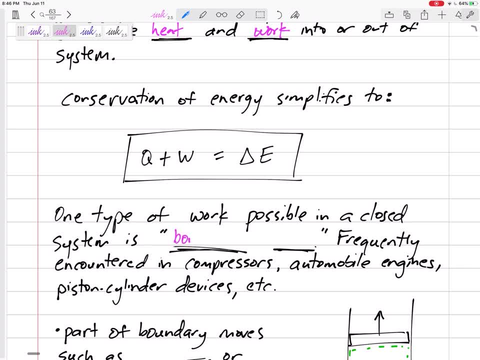 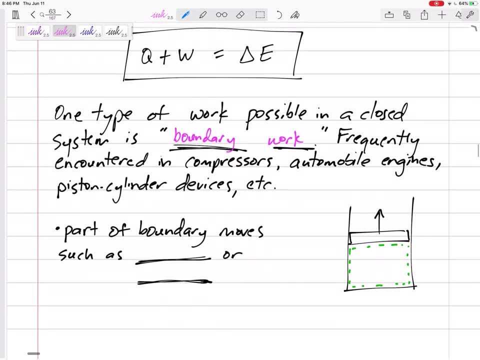 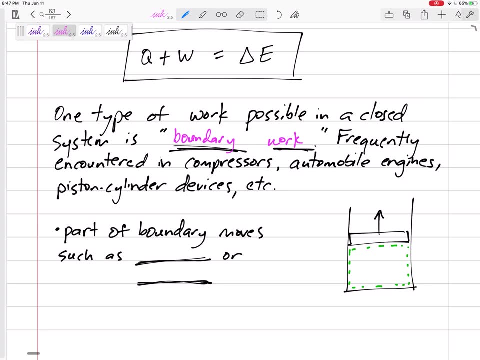 All about boundary. One type of work possible in a closed system is boundary work, Boundary work- and we'll see it in compressors, engines, piston cylinder devices. it's when the boundary moves all right. So if the boundary is moving, then we might need to worry about boundary work. 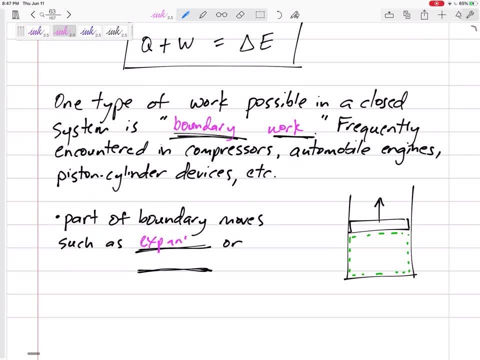 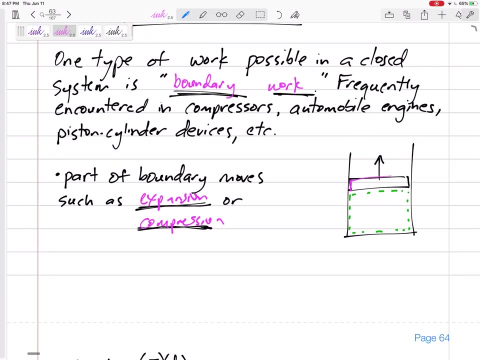 So if we have expansion or compression, if our boundary is, you know, moving, getting larger, if this wall right here- so let's say a piston cylinder device, if we've got some piston right here that is moving up, our boundary is expanding. 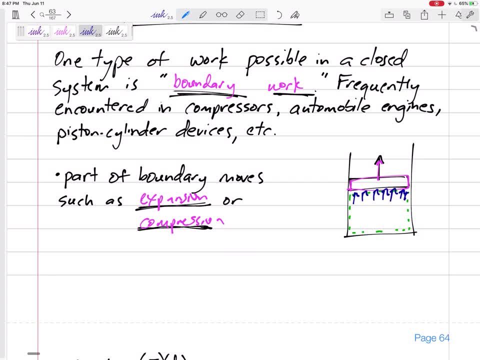 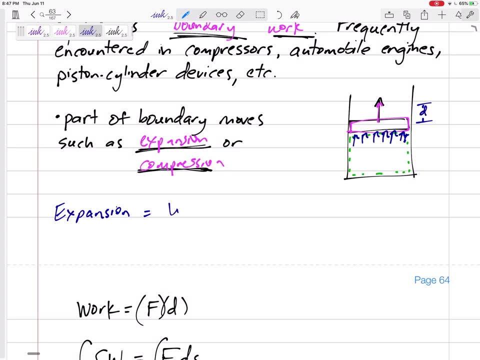 We've got some, you know, pressure that is pushing this and maybe, let's say, this moves a certain distance, and are you seeing some sort of work that might be happening? All right, so an expansion is work out. okay, An expansion is work out. 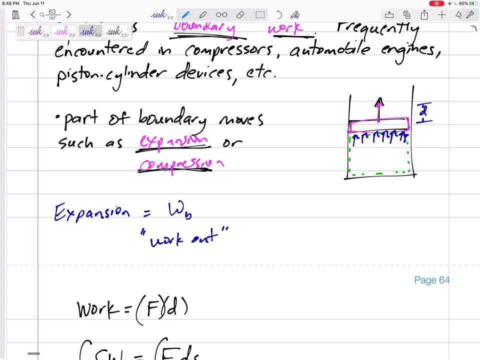 Because it's almost like the system is doing the work right. The fluid is doing the work, Whereas compression it's going to take some outside work. We're going to have to put work into the system to do some compression. So compression is work in. 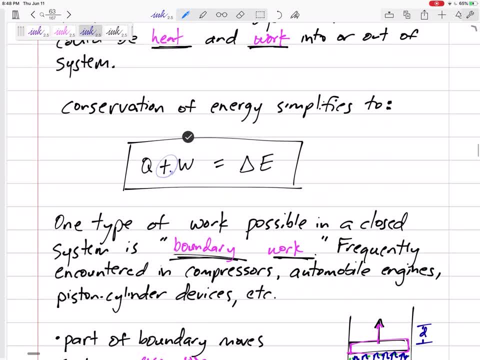 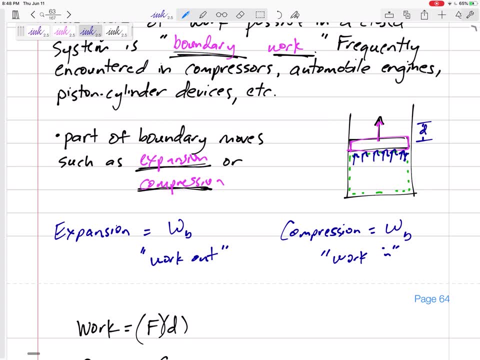 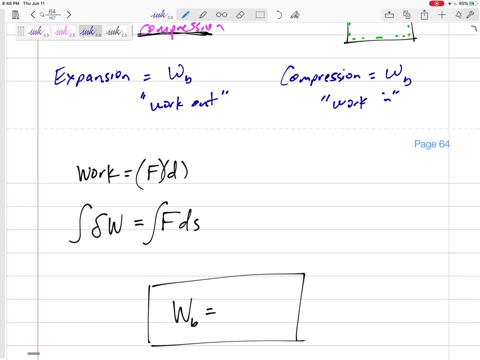 And remember I'm going to say Q plus W and I'm going to say work out is negative, N is positive. right, Yeah, N is positive, Out is negative. Okay, My, I don't know. my high school definition of work is a force times, distance. 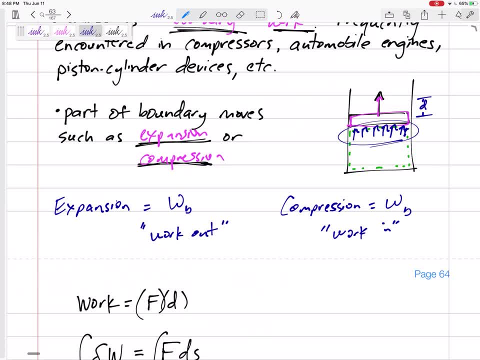 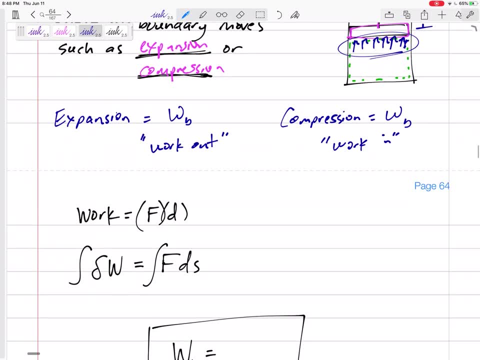 It's almost like we kind of have a force pushing on the boundary and the boundary is going a certain distance. So let's kind of start here. So the work equals force times distance. but a better idea is, like the integral of this: delta W. 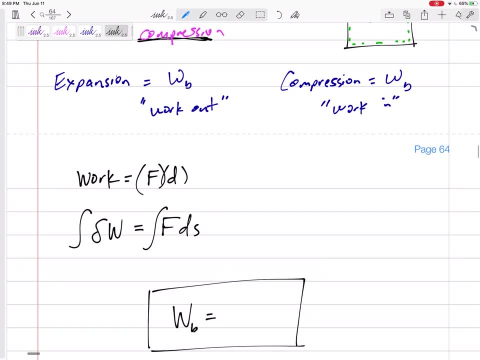 this delta is like a DW. this lowercase delta just means it depends on the path. depends on path, It's a path-dependent integral. So anyway, the work on the left-hand side is equal to if we don't just have one constant force, that's going a distance. 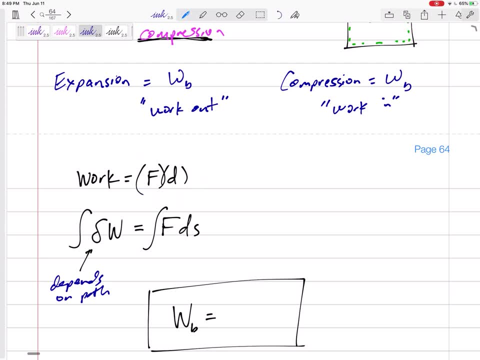 that's in the direction of the displacement, that's in the direction of the force, then we should really do an integral of FU, Okay, Okay, DS, all right, and a force kind of like here. what if we have a pressure instead of a force, right? 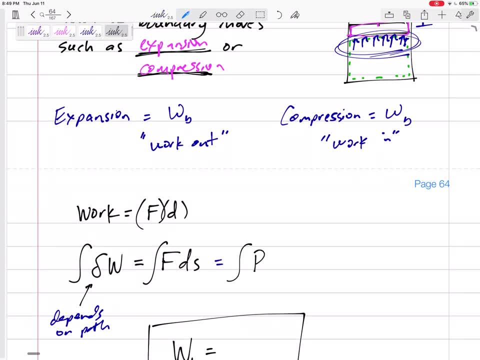 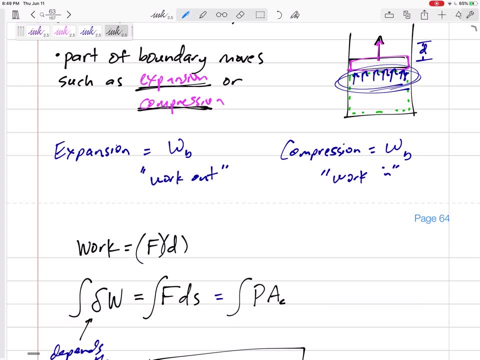 What if we have a pressure instead of a force? then maybe we could say this pressure times area right here, this might be like the cross-sectional area of this, of this face right here, DS. So it's really the integral of PADS and this cross-sectional area and this DS. 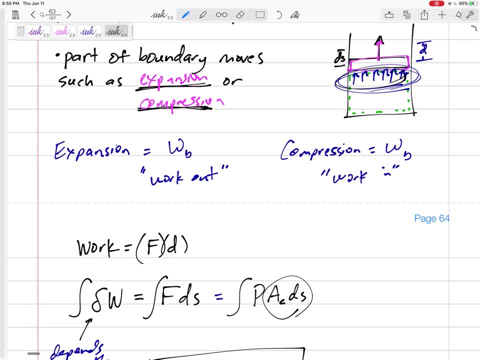 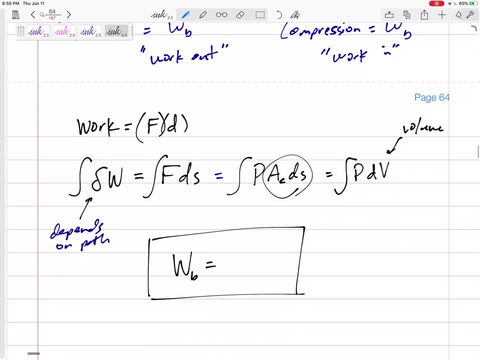 this is a infinitesimally small distance S that it is moving. that is DV, right? Does that make sense? that it's DV a differential volume, That V is volume not velocity. So the work right here, left-hand side of our equation, the work right, the integral of a delta. 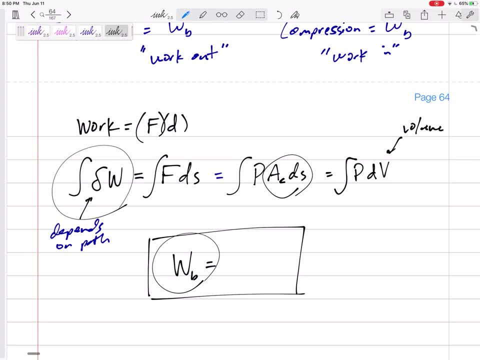 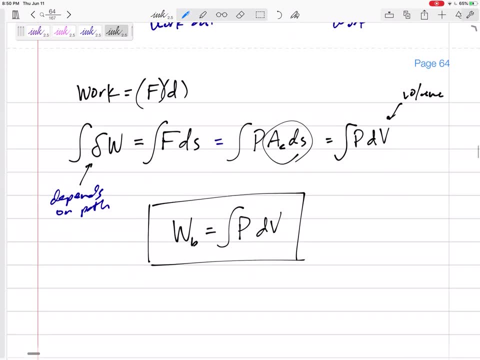 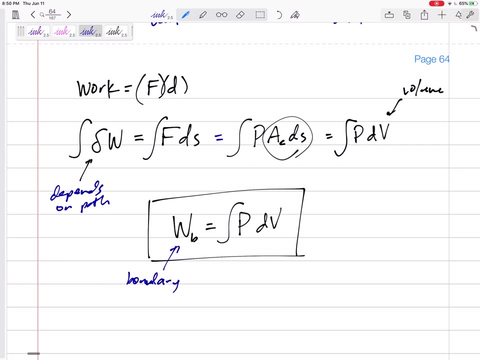 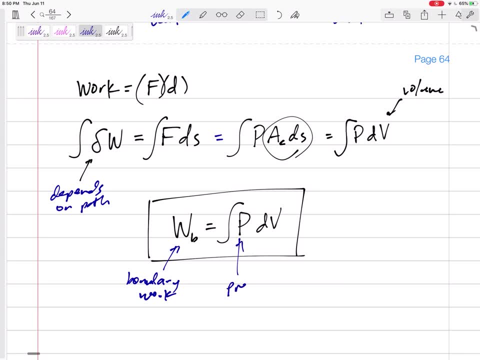 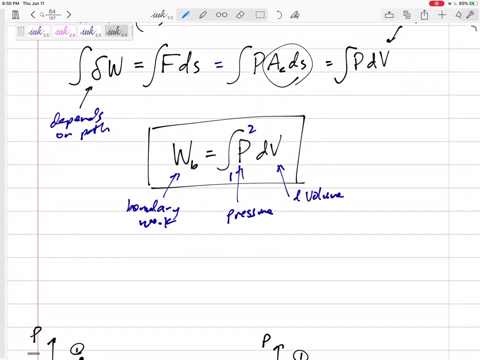 is the integral of pressure times DV, this differential volume from 1 to 2, from 1 to 2.. Let's write that in words: This boundary work is the integral of the pressure with respect to, or integrating it with respect to, volume, from 0.1 to 0.2.. 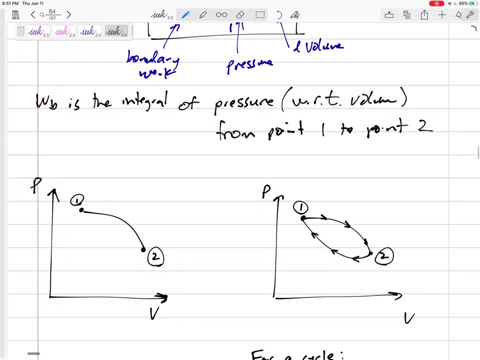 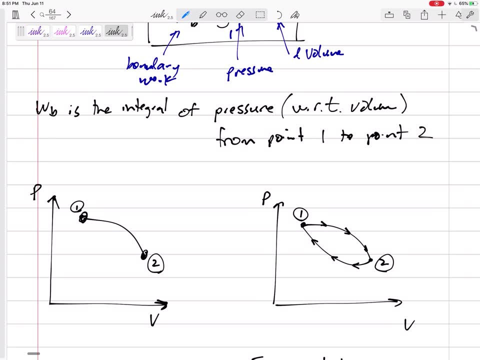 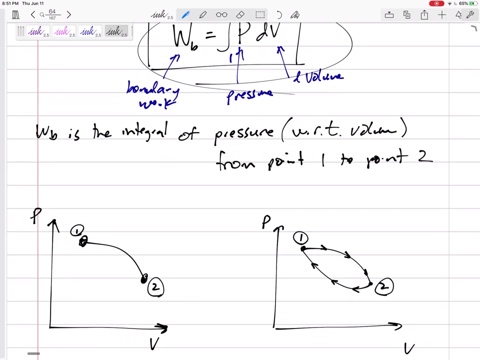 Okay, so what if we could plot the pressure versus the volume right? What if we could plot the pressure versus the volume? and let's say we go from 0.1, right here to 0.2, and we pass all of these different states from state 1 to state 2, what would the integral of P DV B on this PV curve? what would the integral of on this PV curve? it would be the area under this PV curve. 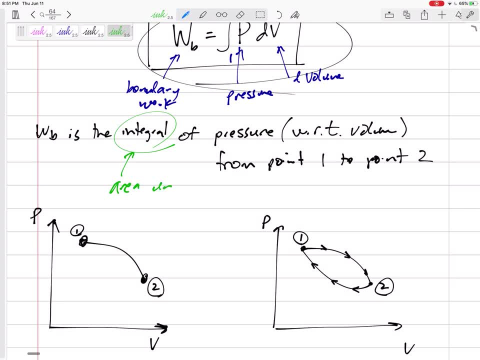 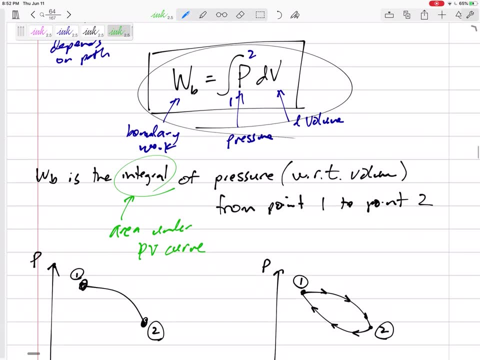 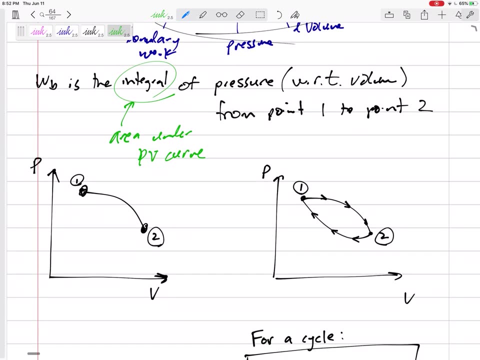 Okay, Okay, Integral is the area under my PV curve. So you know, if we had a function for P then we could integrate it. or if we can kind of plot our P versus V, then we can calculate the area under. 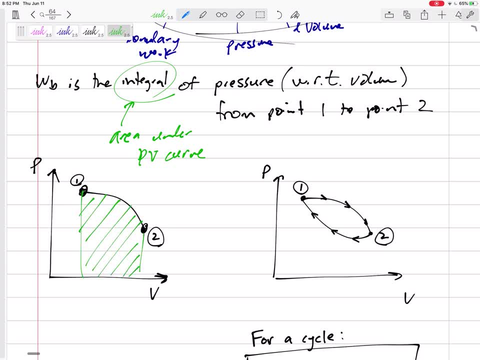 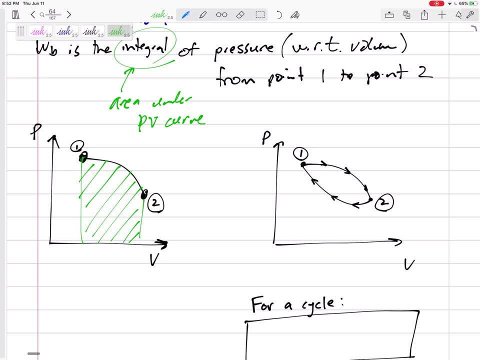 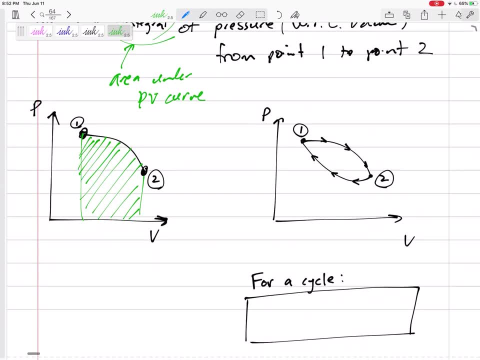 Right, That area. if I can calculate that area, estimate that area or take an integral to find that area, then this area would be the boundary work. This is expansion, Right, This is expansion. Our V is increasing, Our volume is increasing when we're going from state 1 to state 2.. 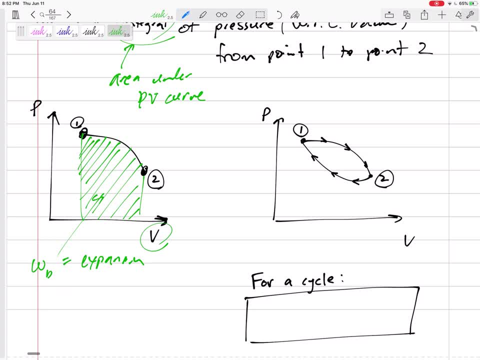 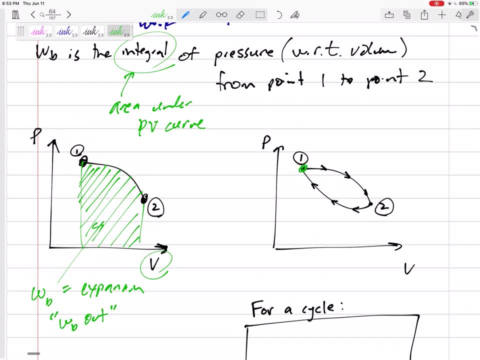 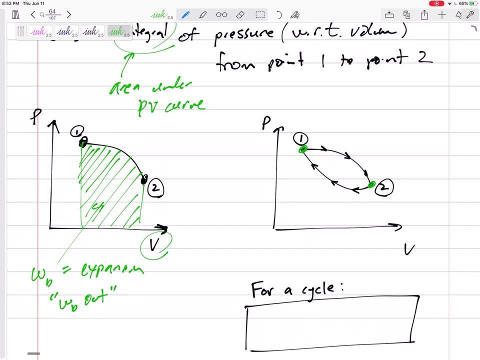 And expansion is work out, WB would be out. okay, alright, let's say, if we, let's say we go from state 1 to state 2 along that path, but we come back along a different path, right, if we go along one path and come back along a different path? 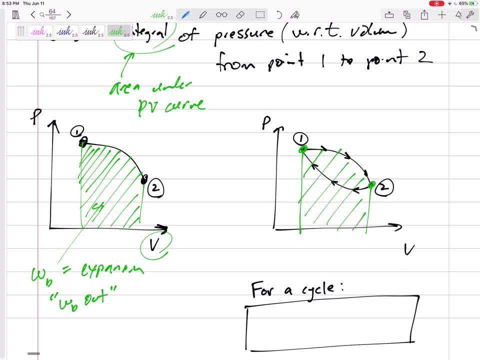 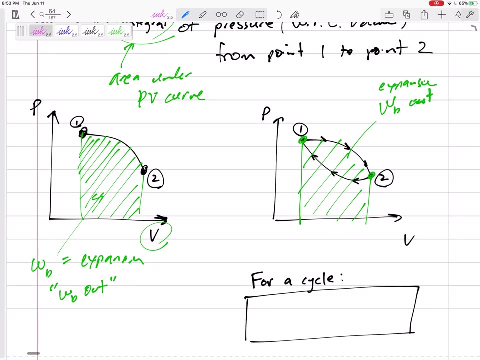 so if we go from state 1 to state 2, that green area would be the boundary work out, that green area would be the expansion boundary work out. but if we come back a different route, a different path, then let's see, this pink area would be.